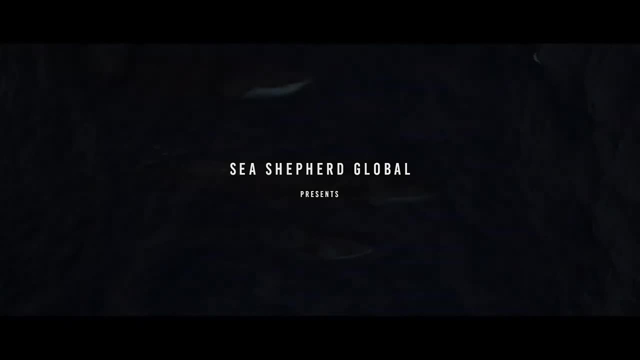 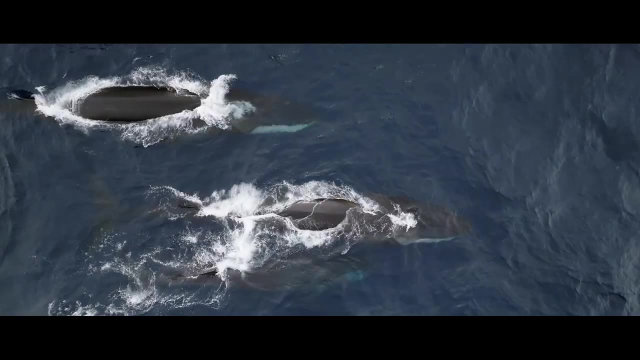 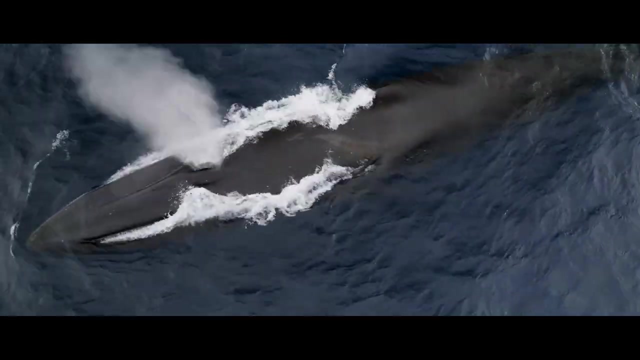 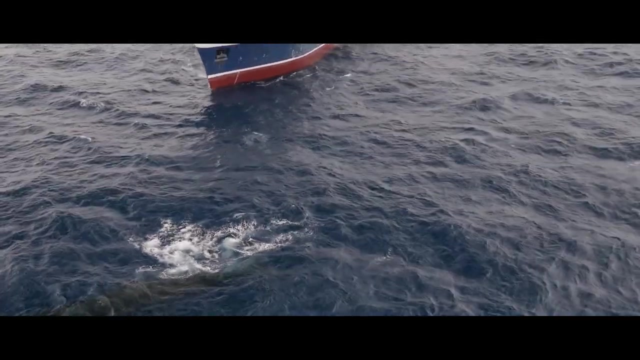 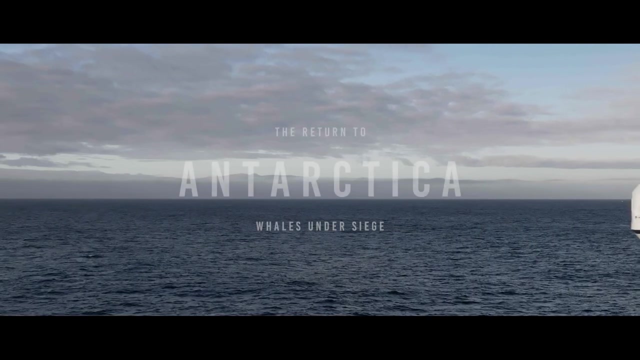 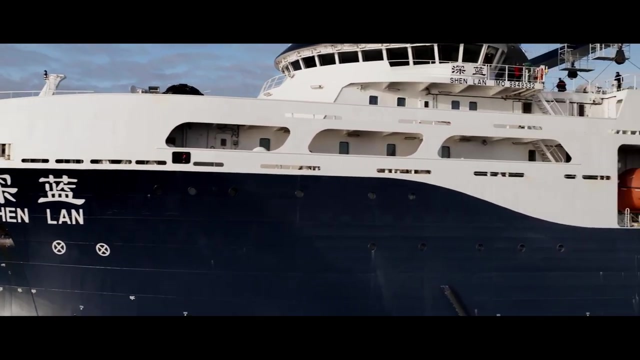 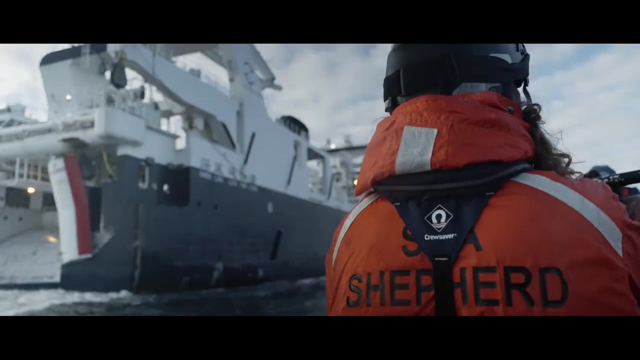 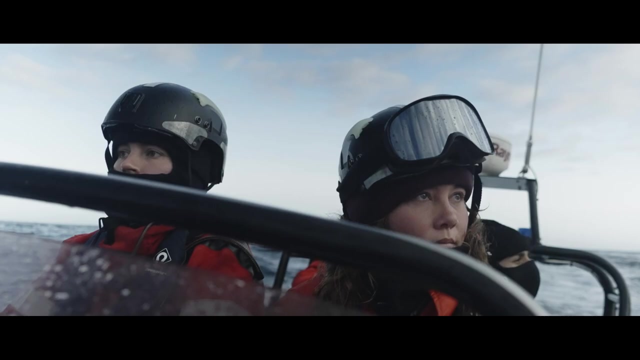 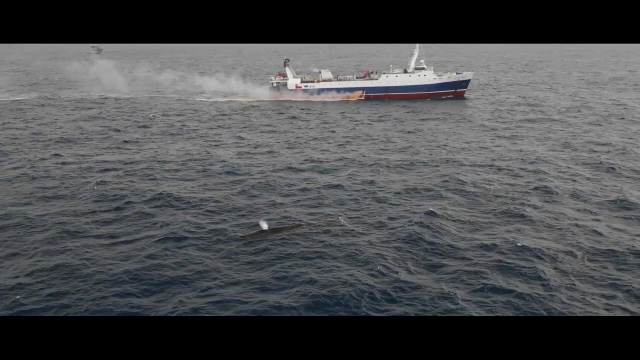 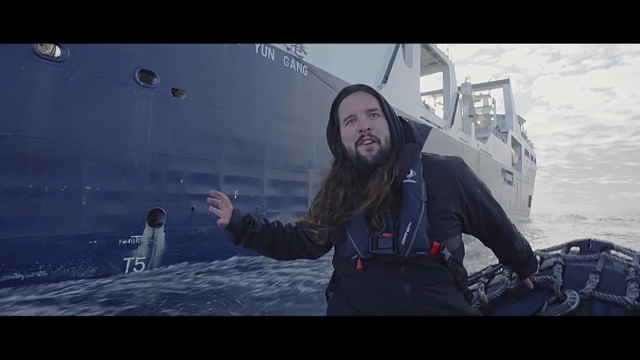 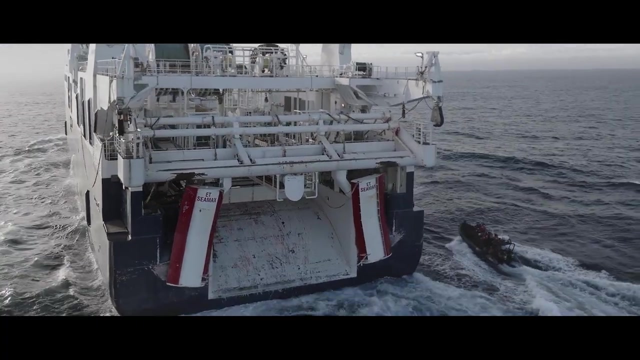 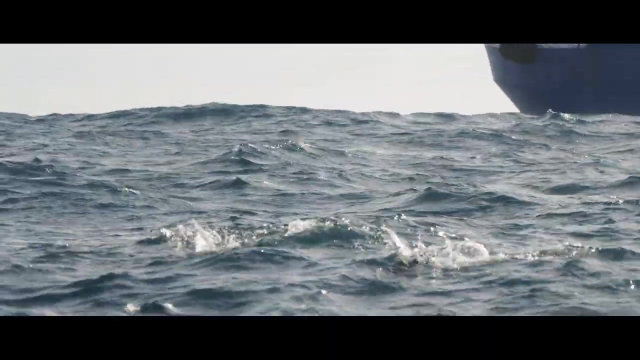 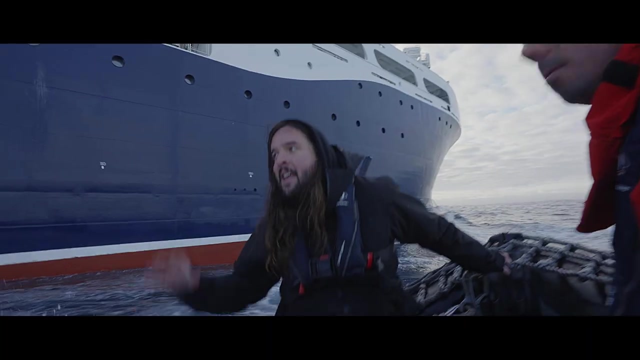 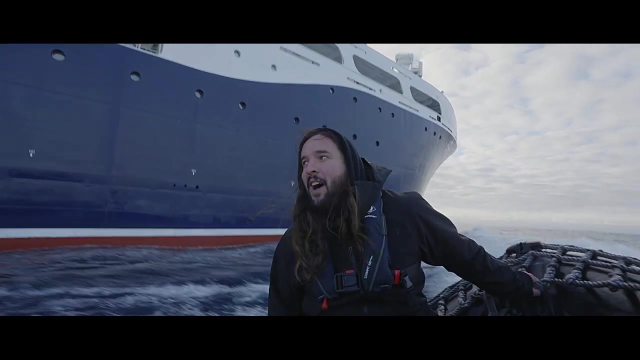 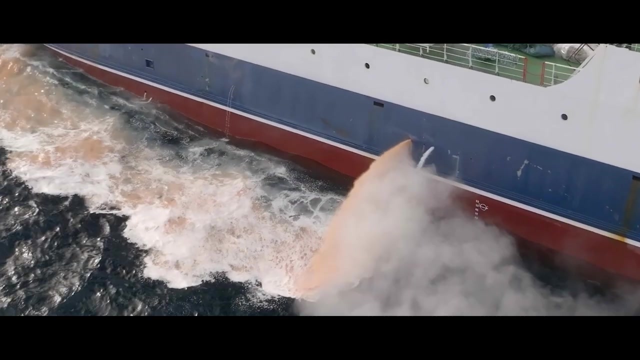 Thank you for watching. Thank you for watching. Thank you for watching These penguins desperately swimming out of the way of this vessel rely on to survive Inside this vessel. the crew will get pulled up the slipway. They'll be cooked or they'll be frozen directly as fish meal. 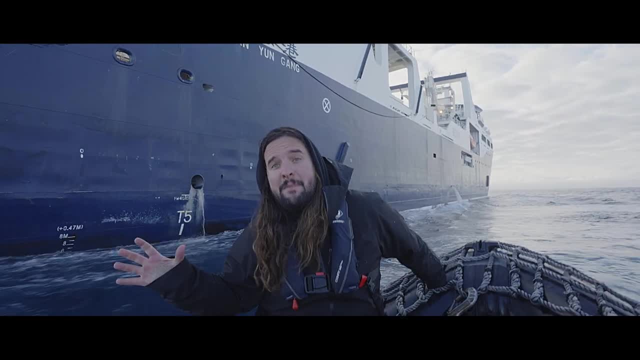 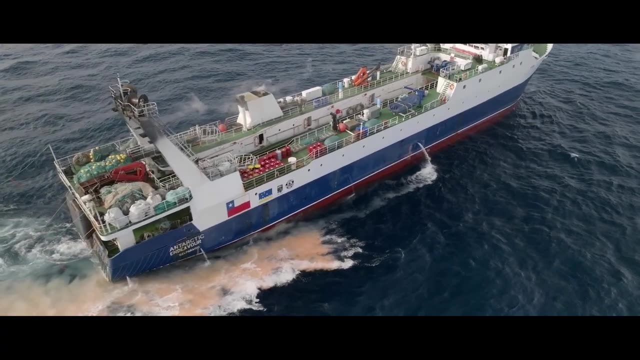 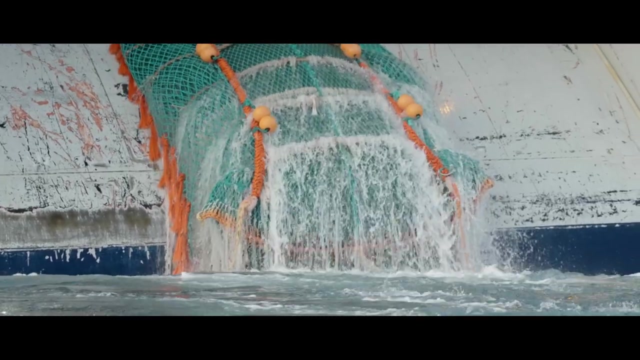 Now the crew is used for fish feed, for aquaculture, to turn farm salmon pink and also for supposed health supplements as part of the nutraceutical industry. This is the foundation of the Antarctic ecosystem getting pulled out of the ocean for products that we do not need. 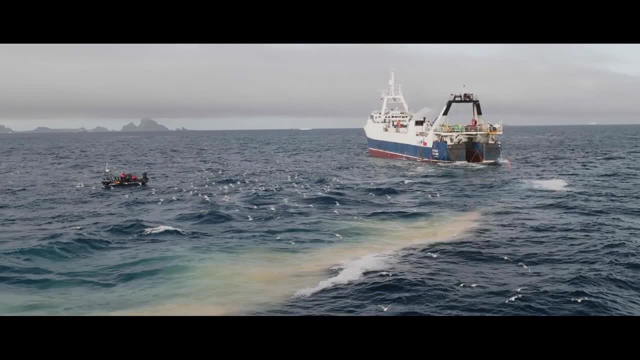 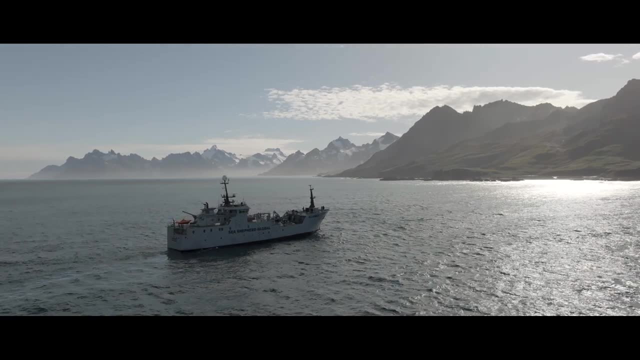 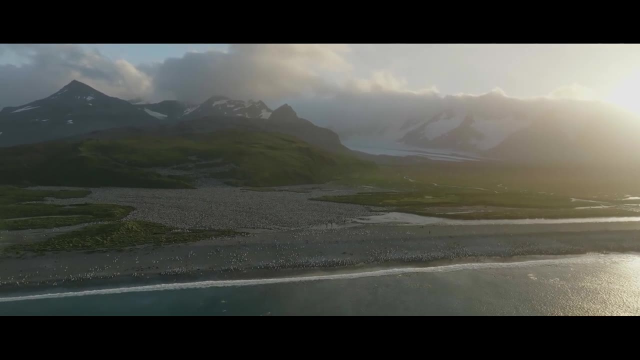 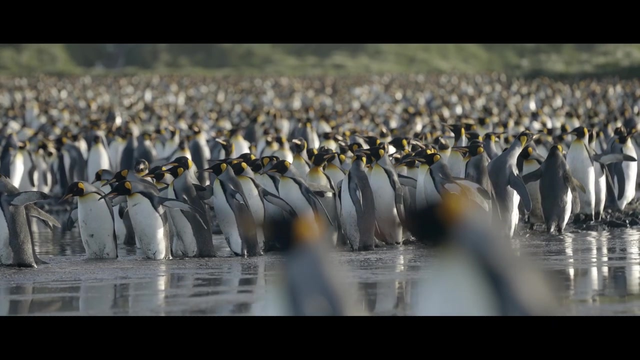 This is the foundation of the Antarctic ecosystem getting pulled out of the ocean for products that we do not need. This is the foundation of the Antarctic ecosystem: getting pulled out of the ocean for products that we do not need. Thank you for watching. 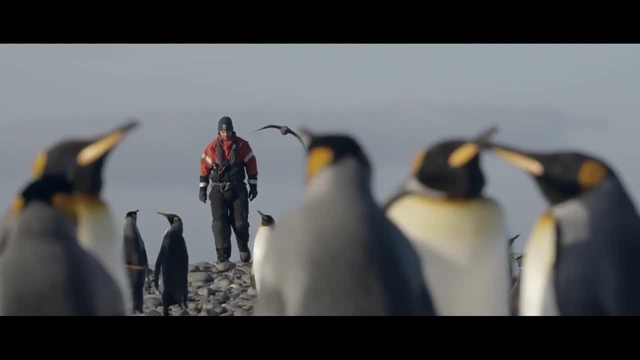 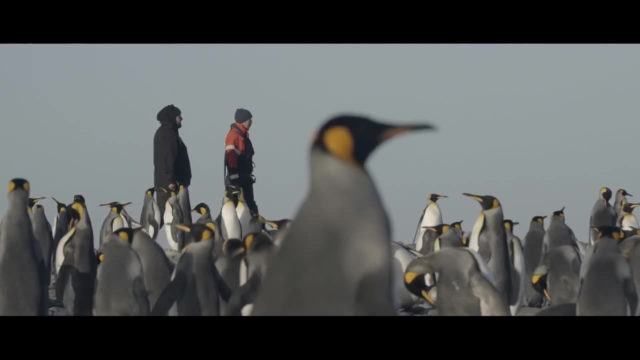 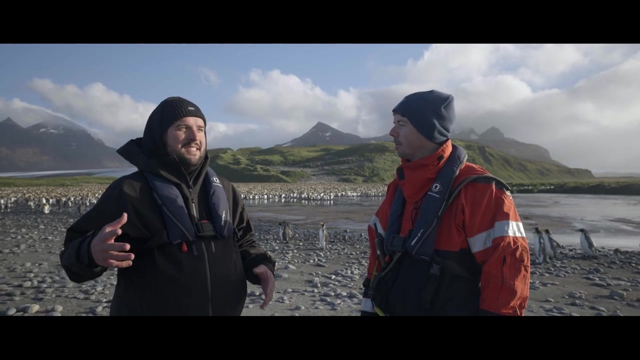 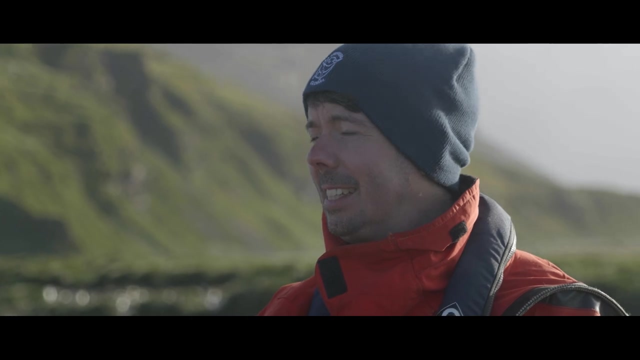 This is really like arriving in another world. When my boot first hit the shore, I was really overwhelmed with the sensation of arriving on another planet, or even the moon. I think it's apt to think of it like a lunar landscape, because I see it like the near side. 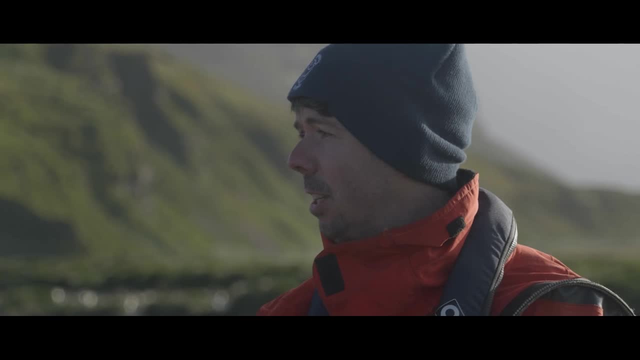 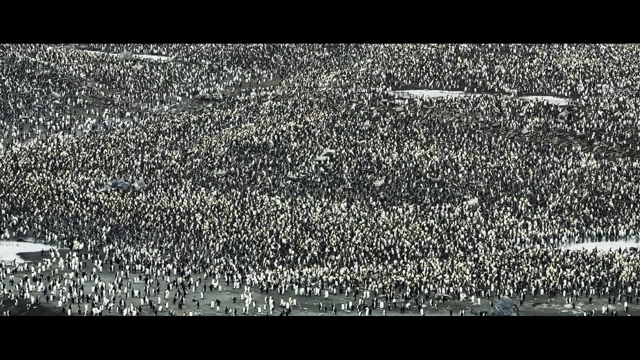 of the moon, right, The near side of the moon that people see every single night, the one that ancient astronomers thought was covered in lunar lakes, And yet on the far side of the moon, the side we don't see, it's beaten and battered. 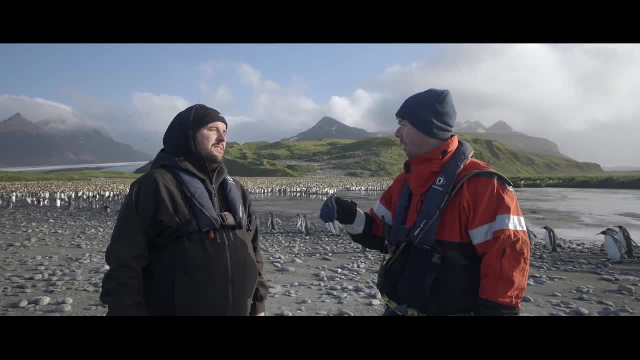 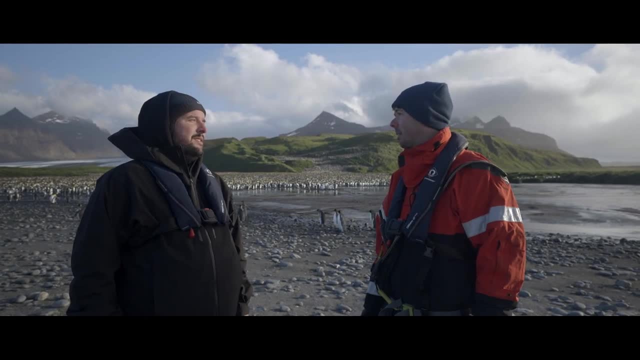 and cratered. There's a dark side to the moon and to fully understand the Southern Ocean, you have to travel to the dark side of the Antarctic and shine a light on the threats This penguin colony behind me here. even though they don't directly rely on krill, they're 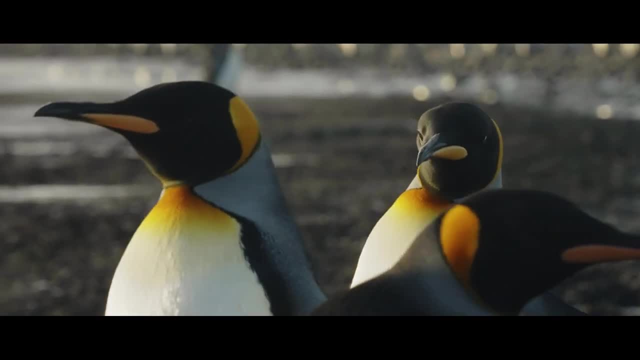 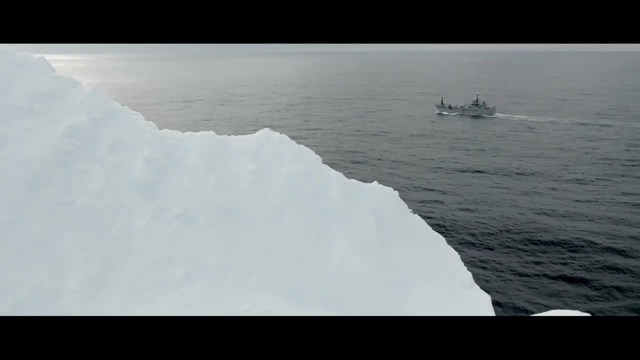 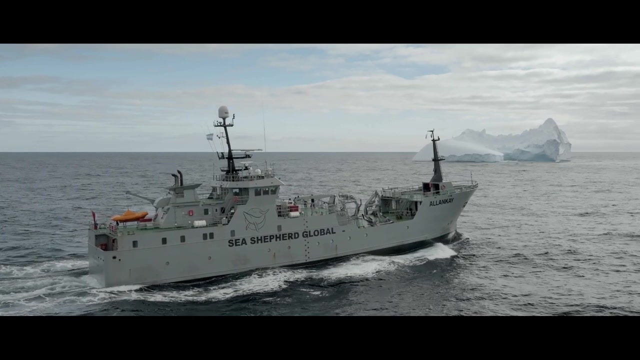 only one or two steps removed. Krill are the foundation. They're the foundation of the Antarctic ecosystem And the krill industry is here hoovering this foundational species out of the ocean. We're just northwest of Coronation Island, where we've snuck up on the long fa. 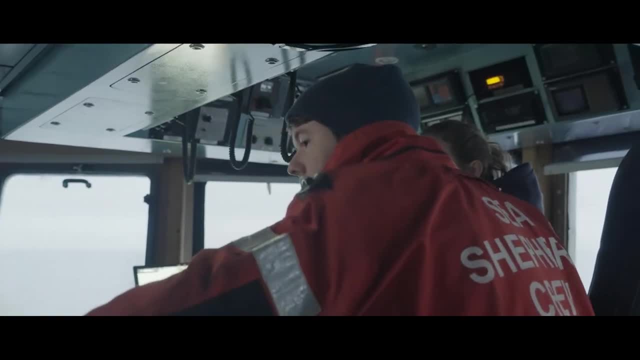 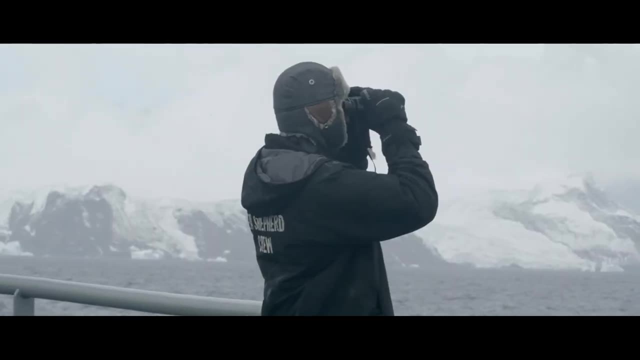 The long fa is part of the Chinese distant water fishing fleet fishing for krill down here in the Antarctic, and it's a harbinger of things to come. We're at a real tipping point for the industry. Either this fishery is going to remain at 12 to 15 years, or it's going to stay at 12. to 15 years. Either this fishery is going to remain at 12 to 14 trawlers or this is just the beginning of what could become a very big fishery down here in the Antarctic. Get the drone up in the air and intercept them as quickly as possible. 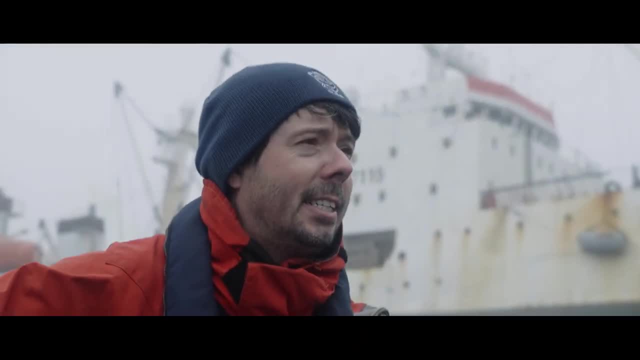 It's illegal to drill for oil in the Antarctic under the Antarctic Treaty System, but there's still oil exploitation happening. It's illegal to drill for oil in the Antarctic under the Antarctic Treaty System, but there's still oil exploitation happening in the Southern Ocean. 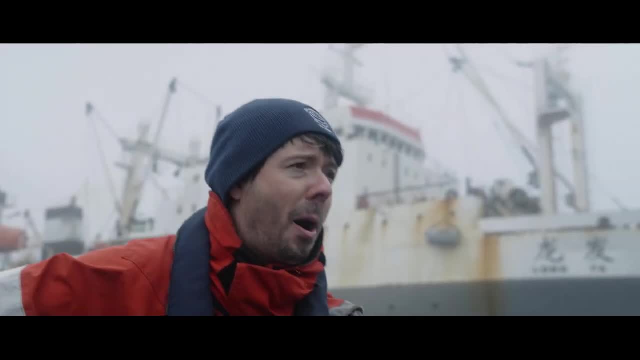 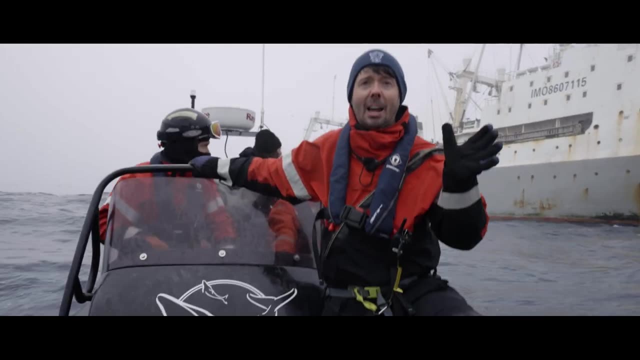 It's just not being taken out of the seabed, it's taken out of the small bodies of krill. In the 1950s, vessels were coming down here to extract oil from the whales. They're now not targeting whales directly, but indirectly, by going after their very food. 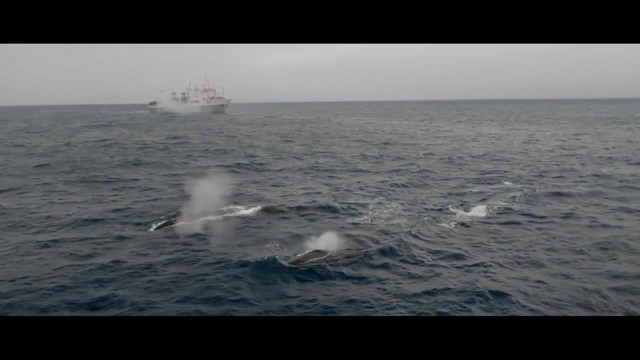 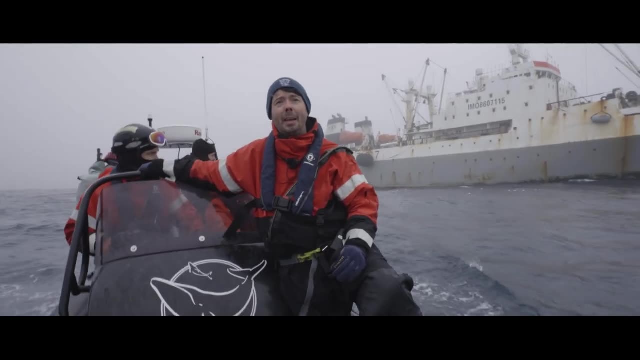 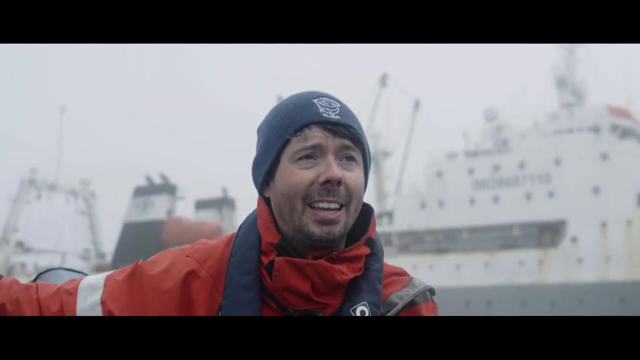 source: The krill fishing industry has long talked about there being a krill surplus, but that only existed because whale numbers had been so heavily decimated due to commercial whaling that some of the great whale species almost went extinct. Whale numbers are now increasing, and if whales were at their pre-whaling number there, 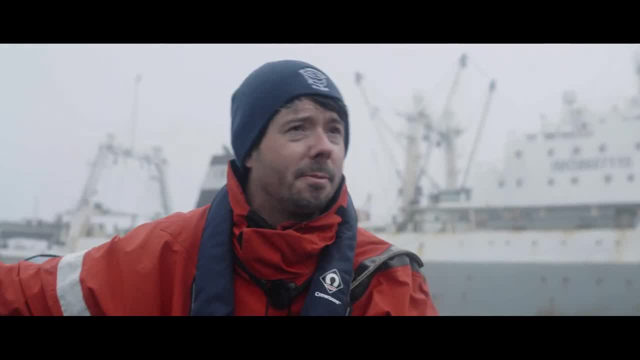 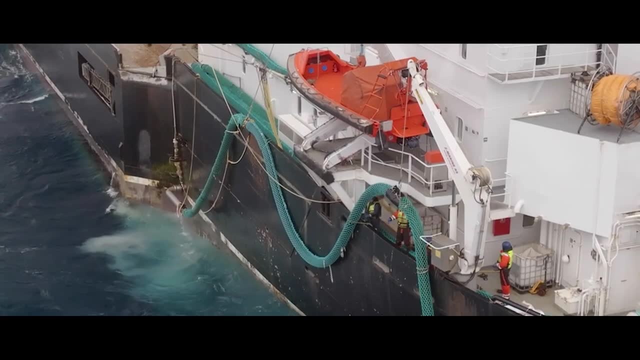 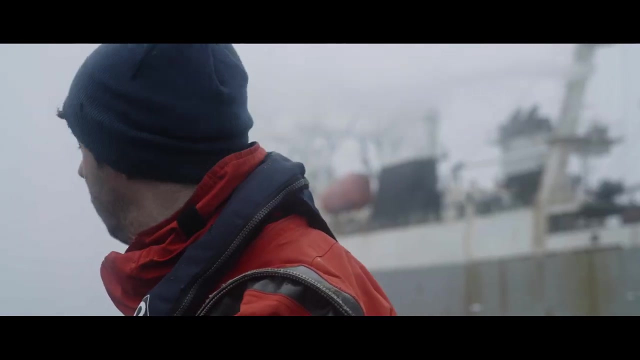 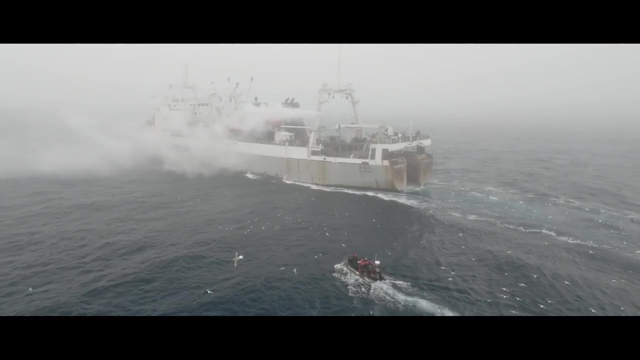 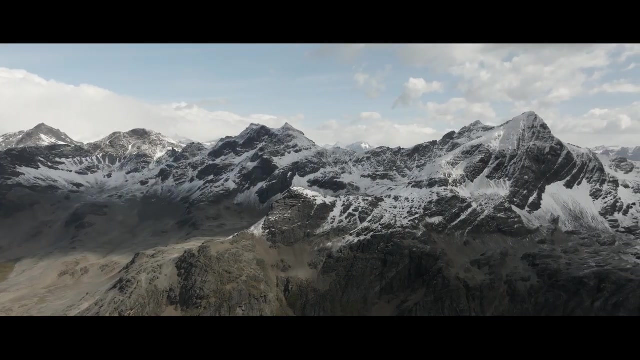 wouldn't be enough krill in the Southern Oceans to sustain those numbers. But it's not all about the history of whale numbers. There's a lot more to it than just from evidence. Some of the world's greatest whale numbers are now just in the virgin.